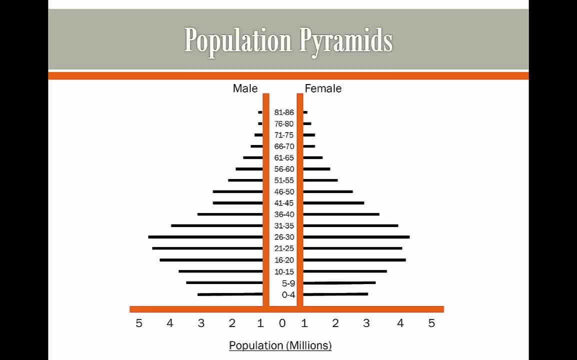 go out either side which indicate how many males and females we have. So let's go and explain it Then. just by running down the middle, we can then see how many of these are actually living in the country in millions. So, for example, if we begin with a zero to four age group, we can have a look. 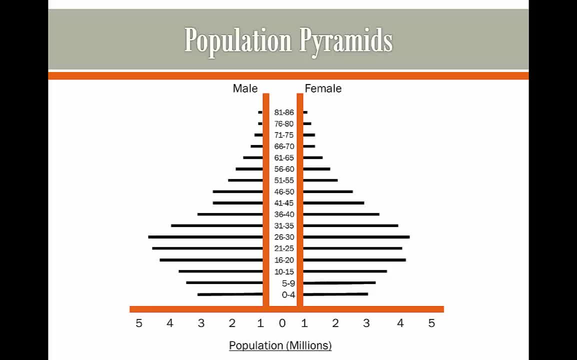 and see that on the female side there's about three million females that are of the age between zero and four in whatever hypothetical country this population pyramid is from. Then we can have a look at the male side on the left and see that maybe it's a little bit more than 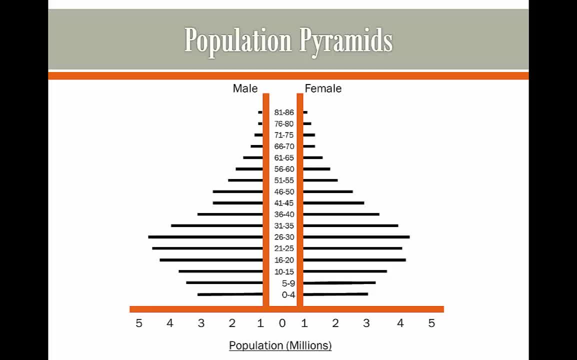 three million, maybe 3.1 million males are between zero and four. So this can. population sort of shape can change depending on the country. In developing countries there tends to be more people along the lower end of the spectrum, say the bigger numbers in the zero to four to ten to. 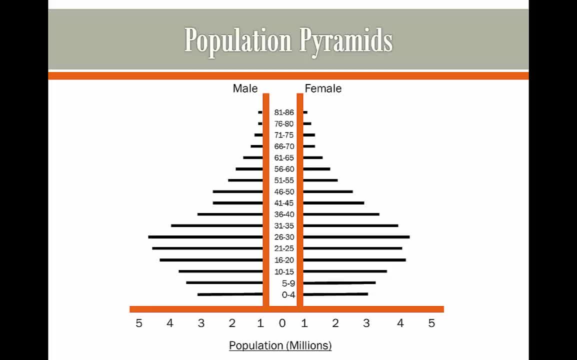 fifteen ranges and much smaller numbers in the sort of sixties and seventies. This is simply because life expectancy is so much shorter and in developing it will. in developed countries, where life expectancy is longer because of better sanitation, health care, etc. There are a lot more. 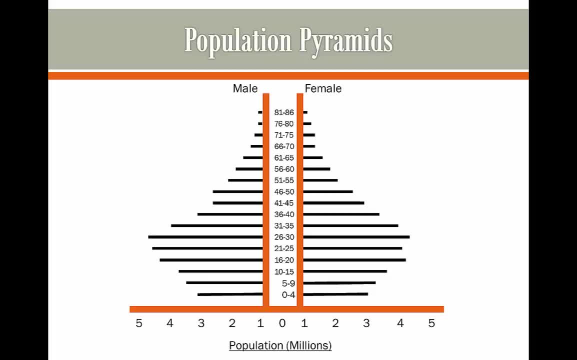 people that are quite older. we tend to see more 40 year olds, 50 year olds and 60 year olds and a lot less sort of children and teenagers, simply because people have already had their children and the population is aging and not many more young people are coming into the country. Now we're going to 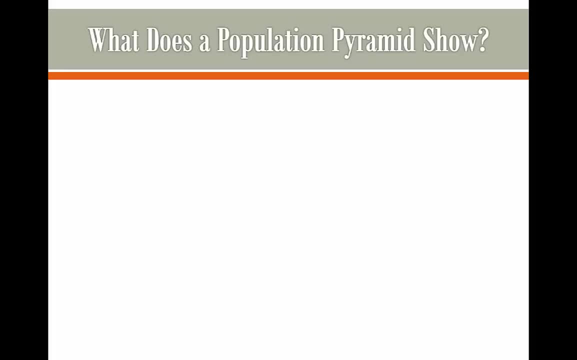 see what population pyramids can show, just apart from sort of numbers and stats. By looking at population pyramid, we can see that there are a lot of people who are older than them and there are a lot of people who are older than them, and there are a lot of people who are older than them. and 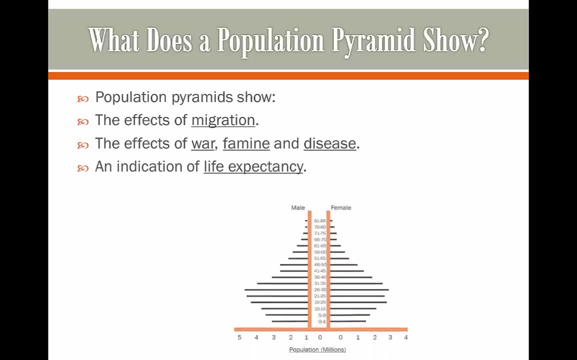 an indication of life expectancy. So let's take this population pyramid as an example. we could probably tell if there has been a lot of migration in the country, because when people migrate to a country, the main reason they do so is looking for work. This means that the people are probably going. 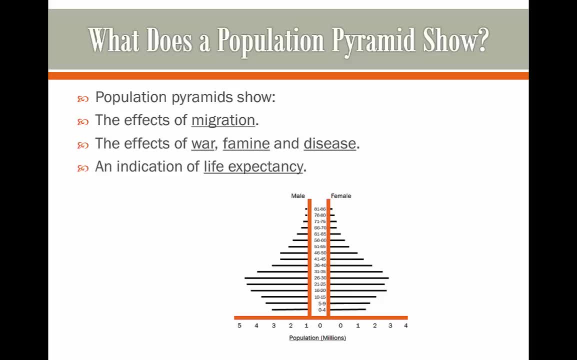 to be aged between their twenties and thirties. So if we see a huge sort of boom coming out from that age range in a population pyramid, we're going to see a lot of people who are older than them and we can pretty much almost confirm theoretically that there was a lot of migrants coming into the. 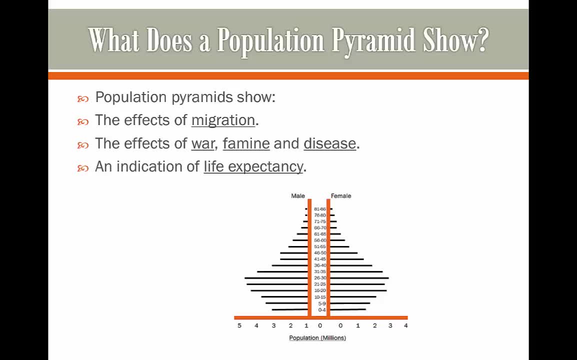 country to try and look for jobs because of that demographic. We can also see the effects of war, famine and disease by the shortages and gaps in the population pyramid. War, famine and disease all kill off people. so all of a sudden, if we see an irregularity where numbers all of a sudden drop, 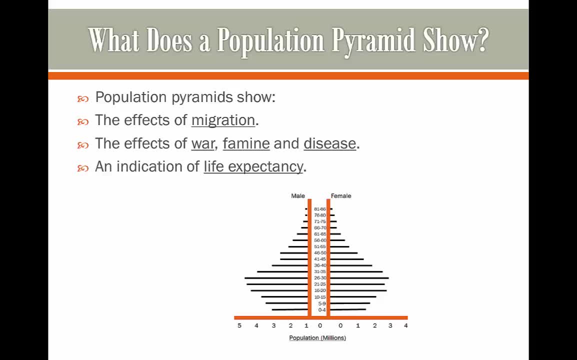 for a certain age range. we can presume that that age group was affected by either war people going off and getting killed, famine people not having, you know, the food to be able to eat and survive, or there could have been a disease that killed them off, such as polio did with a lot of older. 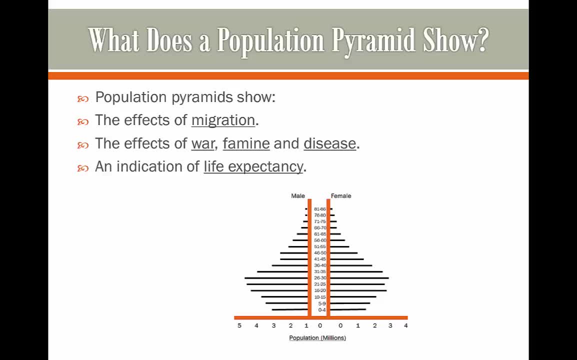 generations Also can show you an indication of life expectancy. If we see a well-rounded number around older populations, we could probably presume that most people only live to that age, and equally with developing countries which have youthful populations, we can tell that because there are so few people. 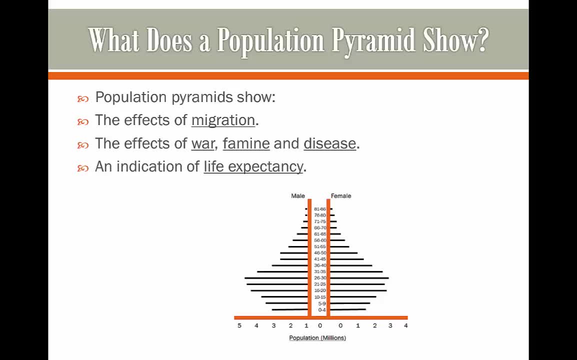 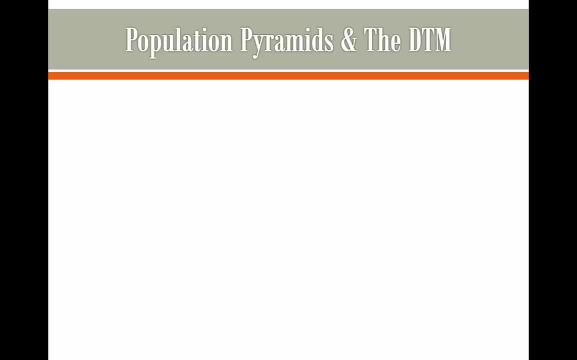 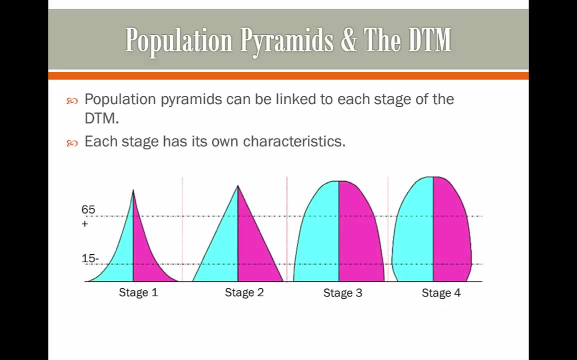 that are in the 80s, mid 70s and mid 60s, that simple life expectancy is not very high at all. Now we can also link population pyramids to the demographic transition model, so each stage is going to have its own characteristics, and here's an example of what the population 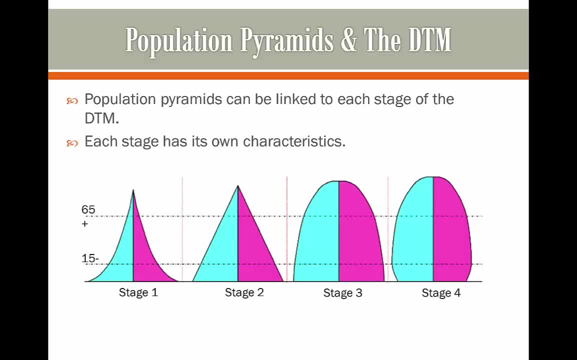 pyramids look like for each stage. In Stage 1, we have a developing country, because it is not very industrialised, not very developed, and because of that there is a youthful population. Check out the video in the description on the demographic transition model if you haven't seen it already, because it would make this. 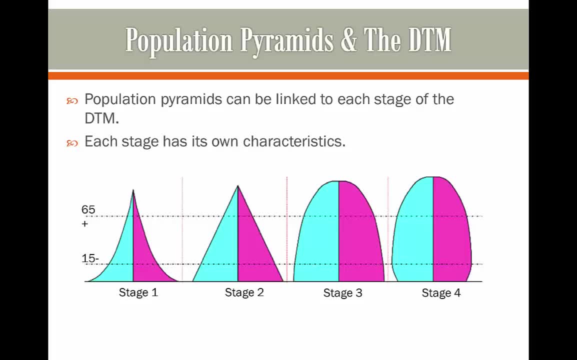 explanation so much clearer Now because the stage one countries aren't very developed. of course they're not going to have a lot of sanitation and healthcare and food, so there are more of a youthful population and less people surviving to live to that older age. Then in stage two countries, 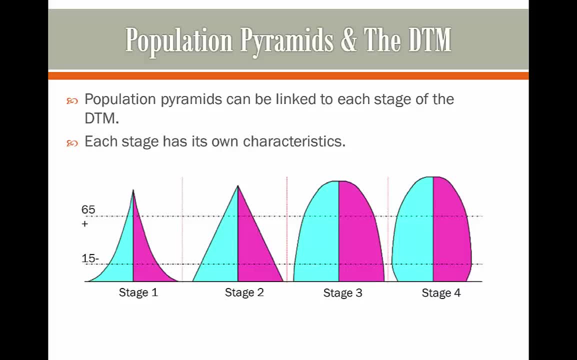 when there's more developed people tend to live longer. so now, instead of a very short older age sort of slumped area, we have a more straightened, more of a regular pattern. Now there are still more people that are being born simply because of lack of education and contraceptions, and you know. 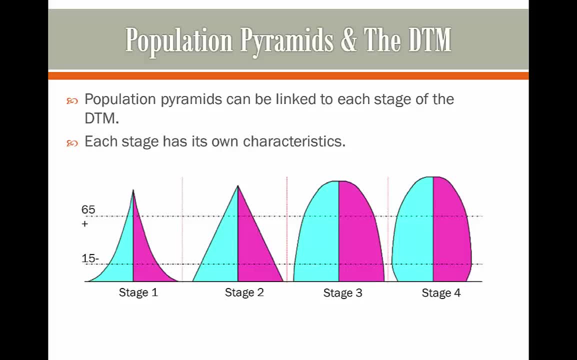 shortage of contraceptions and religious reasons and whatever, There tend to be more youth anyway. so we can clearly see that the base where we have all the youth are much is much greater than all the higher parts of it where we have all the older people. 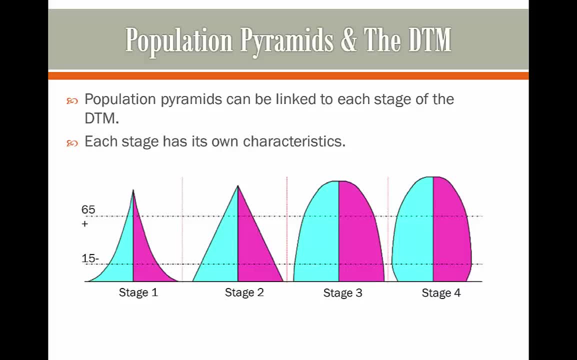 Then in stage three we tend to become more rounded, and this is because the population is kind of becoming more regular. it's not no longer youthful because we now have education on contraceptives and there are more in stock, so the youthful population isn't really a problem. Then in stage four, we 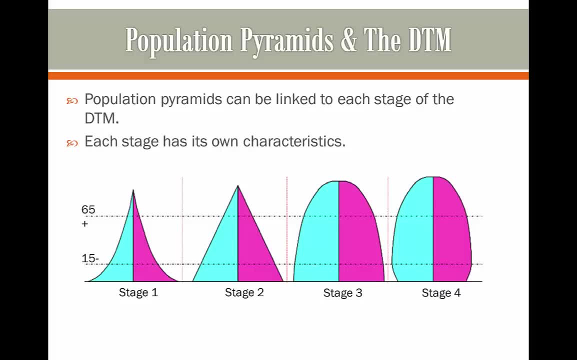 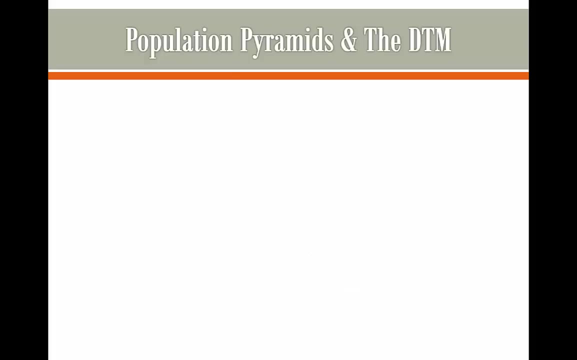 have an aging population, where now we have more old people in the country and less sort of youthful populations, simply because changes in lifestyle and same-sex marriages and different concepts like that. So now we're going to link each stage to the DTM. So here we have our 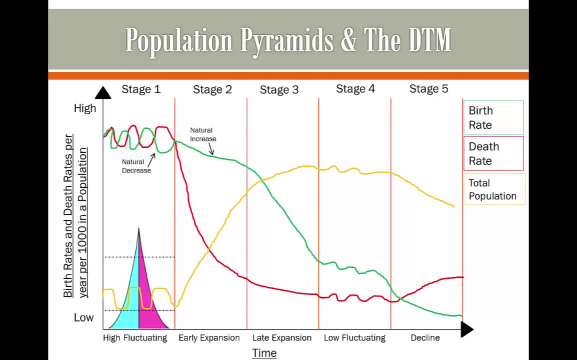 diagram of the DTM. Now stage one can fit on here, stage two, stage three, stage four and now stage five, which we don't have a photo of because technically it's just a theoretical stage. I know Germany may be in it already, but still there isn't really backing to show how population 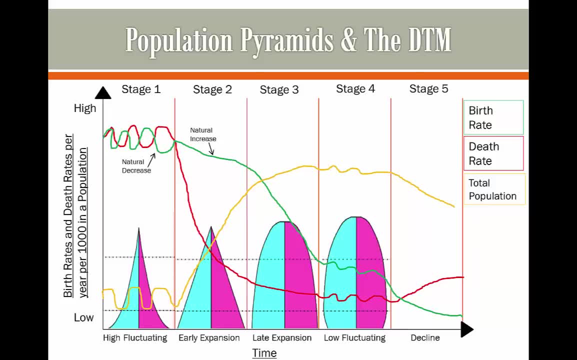 structures can form as part of it, since they look almost the same as stage four. But if we were to draw a hypothetical one on here, we could see that there would be almost no youthful population whatsoever, because people choose not to have all these children, as we can see on the 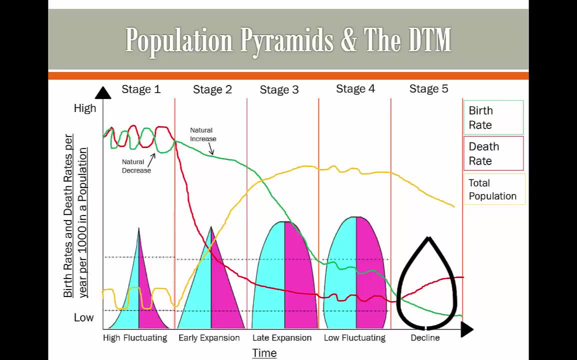 graph because the death rate is higher than the birth rate, And then we have a sort of rounded base where we have 40 year olds- 50 year olds living happily, but then because of the changing lifestyles, the older age then sort of die out as well and we have more of an angular top. 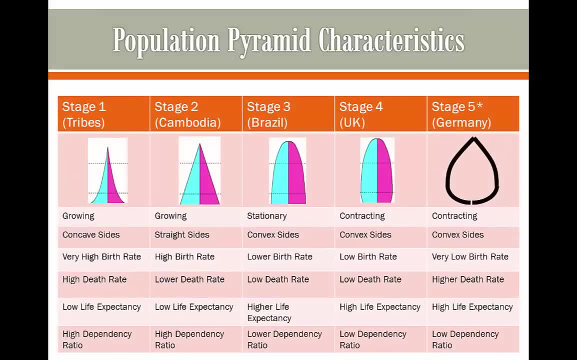 Now we're going to have a look at each characteristic of the population pyramid stages. So hit pause whenever you're ready to be able to copy all these down, because it is a lot of information. but we'll talk through it now quite briefly and quickly, so that you also have time to put it down. So, as we've 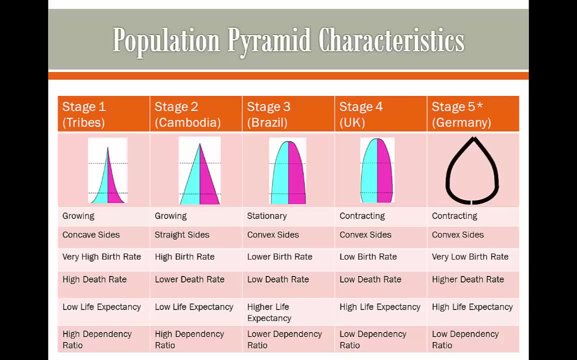 already run through pretty much. we can tell that from stage one, the population pyramid will have a very high birth rate, a high death rate, low life expectancy, but a very high dependency ratio. This is because there are few adults but many children. That is effectively exactly the same for stage two countries where we have an example which is 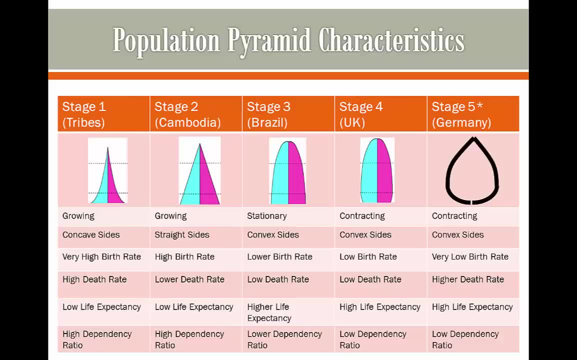 Cambodia. However, this time there are more adults, so the high dependency ratio has actually dropped slightly and also there is a lower death rate due to better developed sort of techniques to deal with death. Then, with stage three countries such as Brazil, we now have a lower dependency ratio. 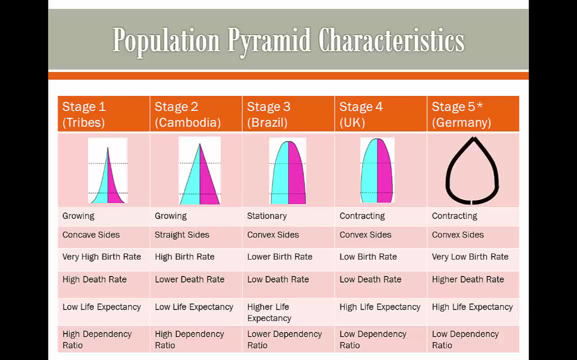 much higher life expectancy and lower death rates. Stage four countries. we have a very low dependency of the population, So we now have a higher life expectancy but we still have a dependency ratio because the bulk of our population is in that working age, and lower death rates as 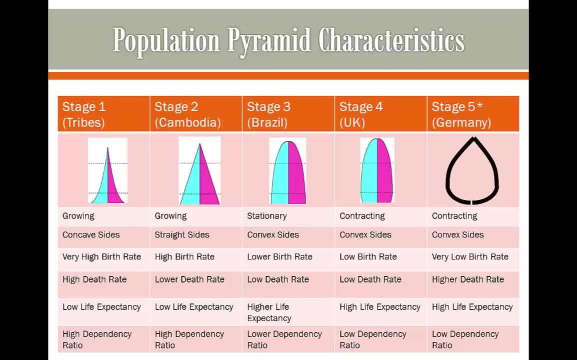 well Then, in our stage 5 country, we have a very, very low dependency ratio because, effectively, the vast majority of the population are all working and there is a high life expectancy, a higher death rate and a very low birth rate, contrary to stage 1 and stage 2.. 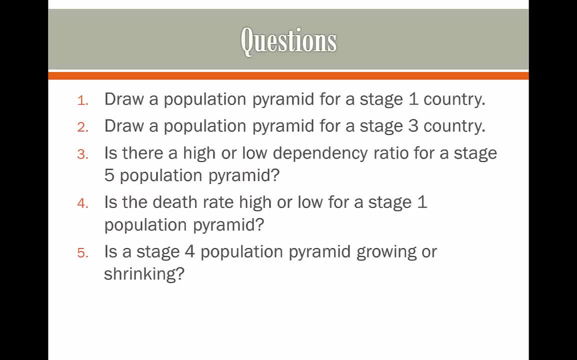 Here you have some questions now on all the information which we've gone through in this video. Hit pause whenever you're ready to attempt all these questions and then you can hit play whenever you're ready to see the answers. Here are the answers, If you got all five of these. 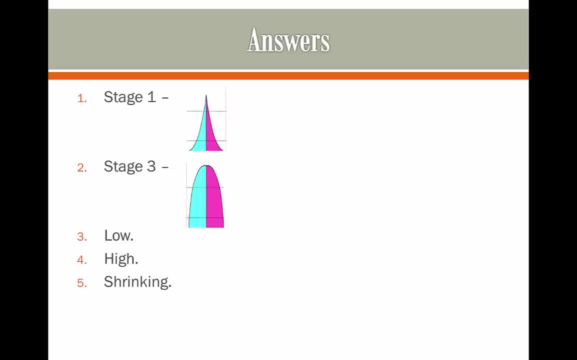 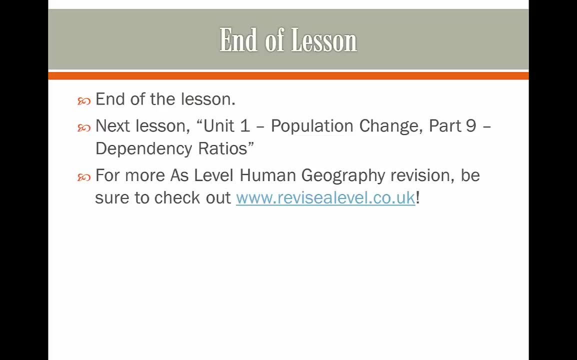 right, congratulations. I would advise you to move on to the next video in the playlist. however, if you did not be sure, to go over your notes once more or rewind the video, or you could check out wwwrevisalevelcouk for some more geography revision. Join us next time where we're going. 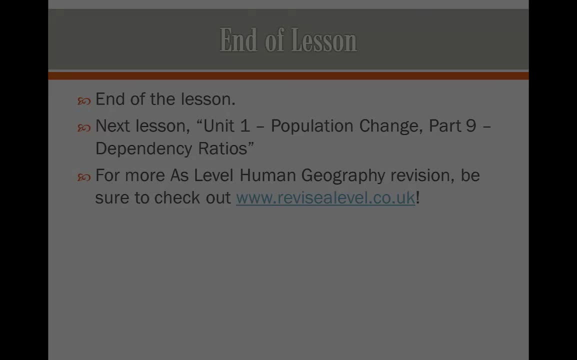 to be looking at dependency ratios. Until then, I will see you in the next video. Thanks for watching. 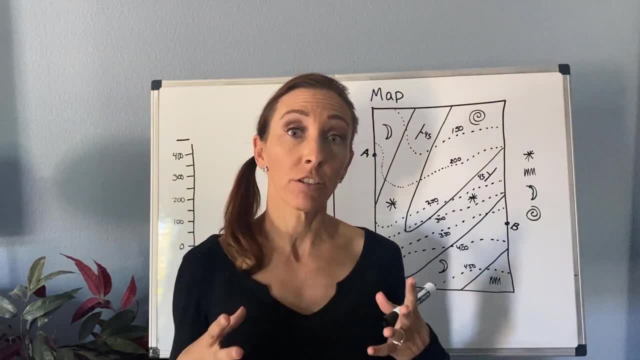 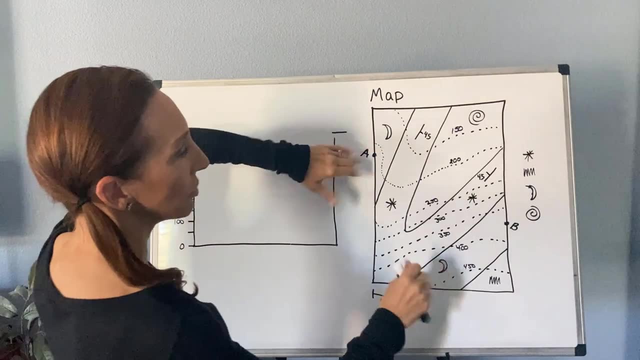 I want to teach you how to construct a geologic cross-section with a topographic profile from a geologic map. So the idea here is that we have a geologic map and if we look at it, a couple things we notice. We have several units marked here and that's in. 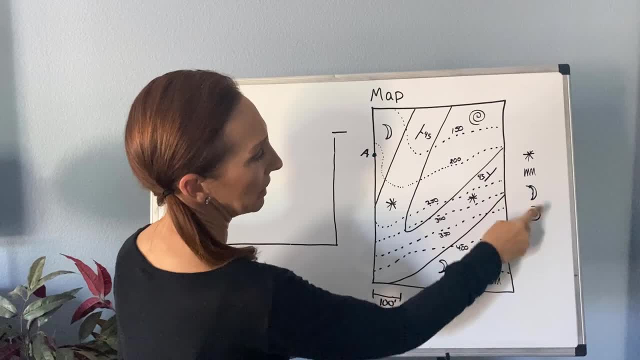 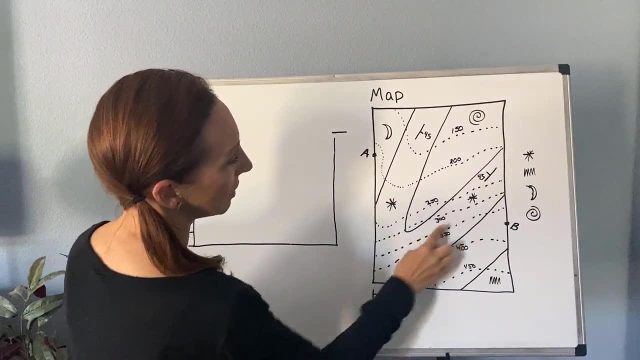 no particular order. So this asterisk, the squiggle, this kind of banana moon shape, and this spiral, And so if we identify those units, we can find the spiral here, here's the asterisk, here's our moon, up here and at the top, and then a little squiggly one down here.